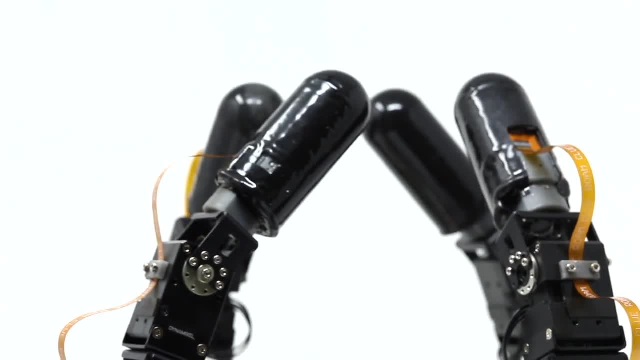 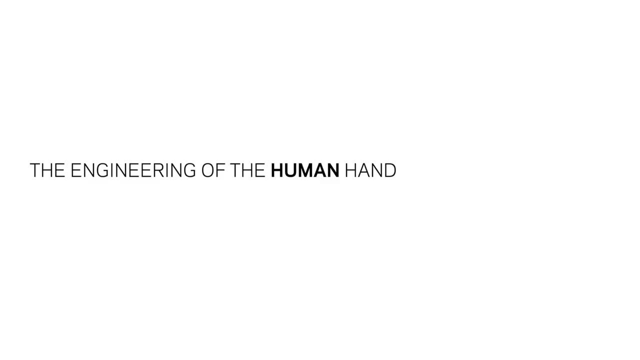 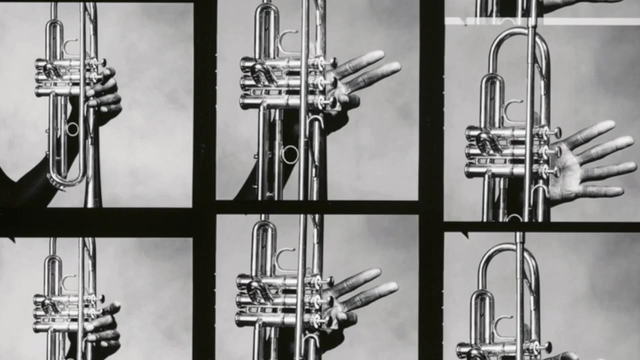 we've been focusing on tactile sense. Tactile sensing is key for embodied physical agents interacting with the world. If you think about the human hand, a marvel of engineering, more than 25 joints, individual degrees of freedom, more than 40 muscles articulating those joints, But then, of course, also the 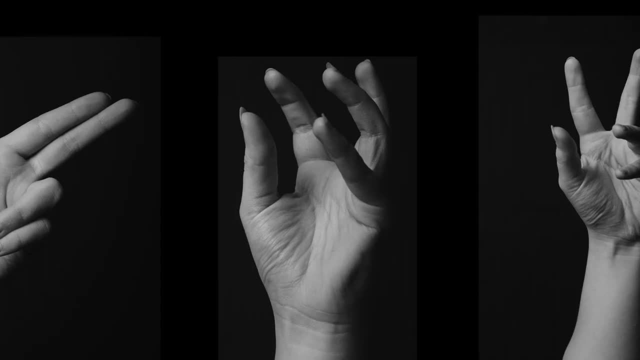 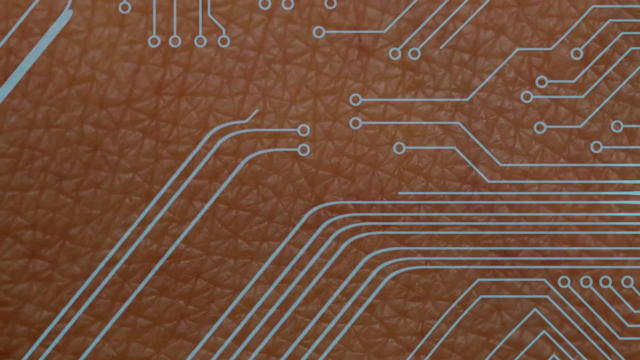 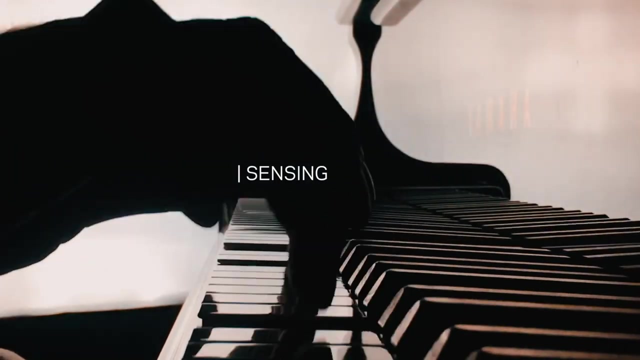 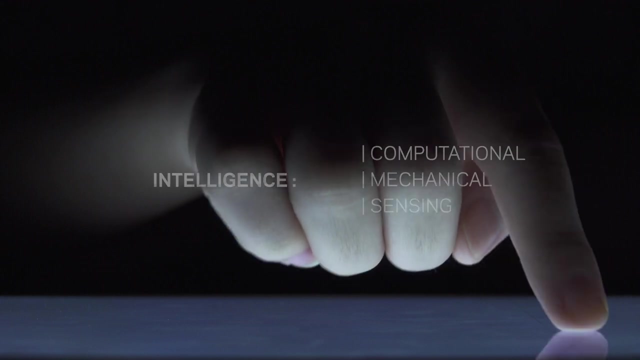 sensing mechanism. We have hundreds of individual mechanoreceptors in each fingertip that are constantly collecting different kinds of information about touch: The computational intelligence, the mechanical intelligence, the sensing intelligence. In biological evolution, all of these components evolve in lockstep together. 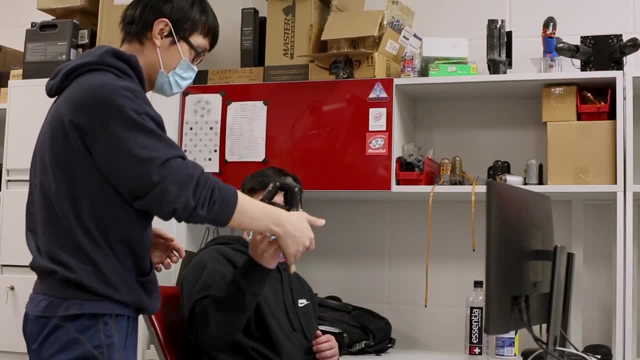 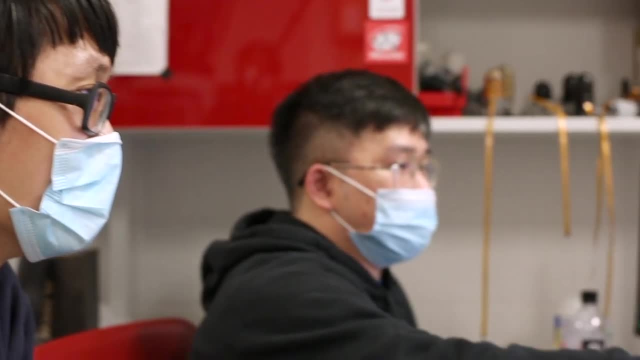 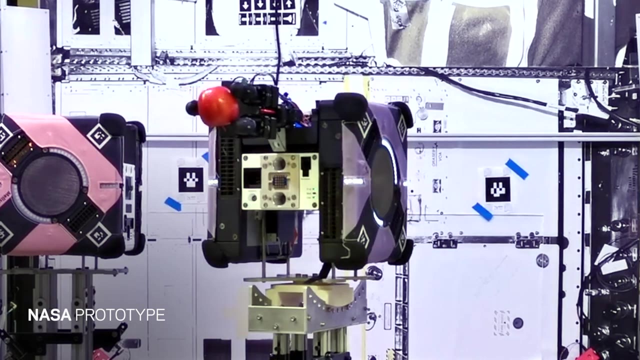 So we've been asking: can we optimize the mechanical design of a robot at the same time as the computational policy with and for each other? And this is where we come to the big, big advances that we've seen in the last five years. 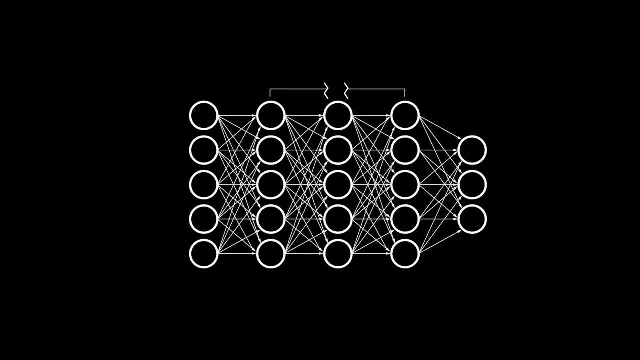 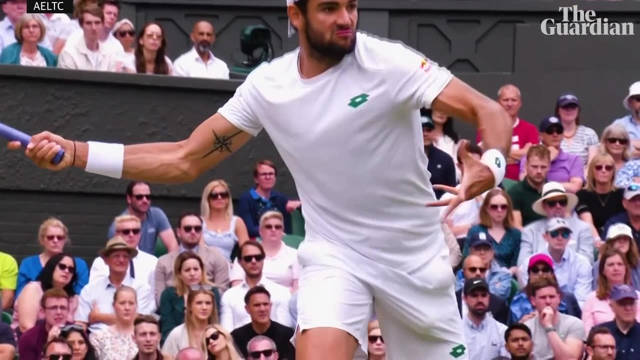 The first is the field of machine learning and reinforcement learning. Some of these modern reinforcement learning techniques are really really well suited for operating in situations where you have imperfect knowledge of the world. You can think of it almost as a muscle memory, right, Every time you hit a tennis ball you don't have perfect knowledge of. 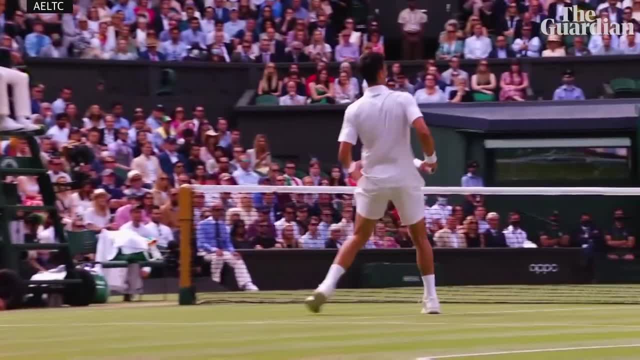 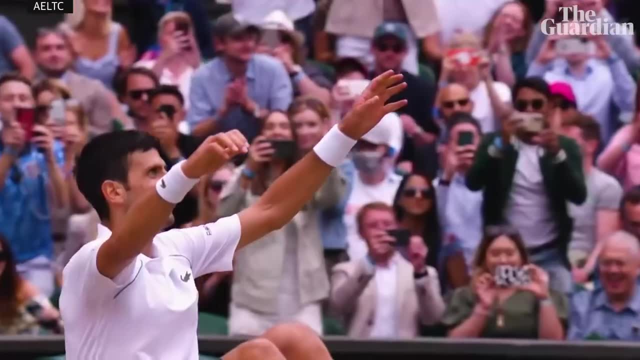 the ball's exact velocity and spin. You get your sensor data which tells you something about the world, and then your muscle memory takes over and says: you know, last time how did the world look like this. These are the actions that I took and things turned. 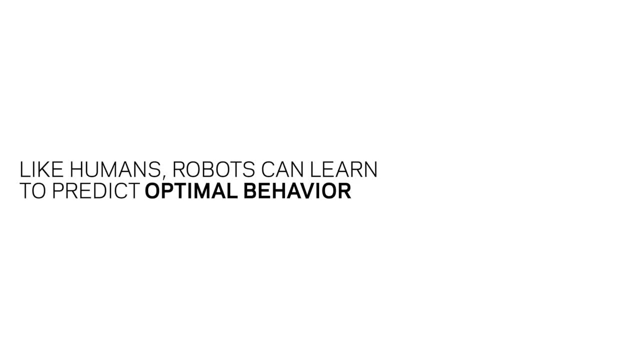 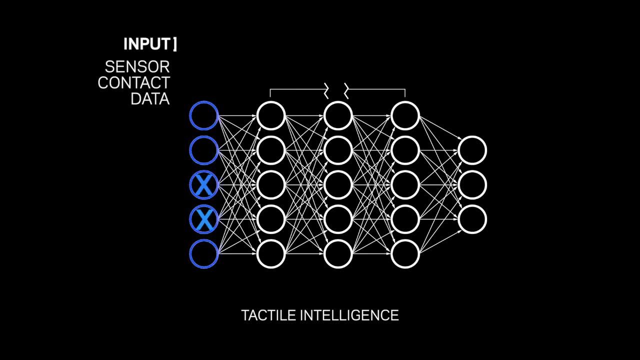 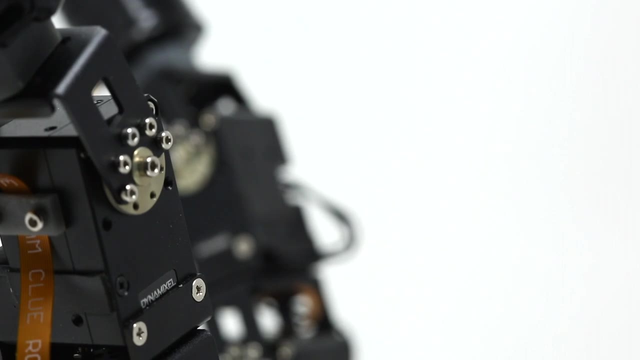 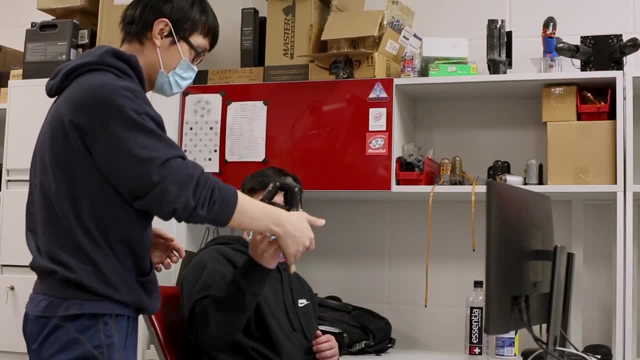 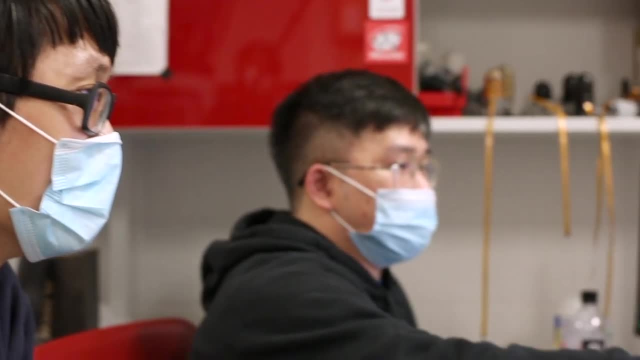 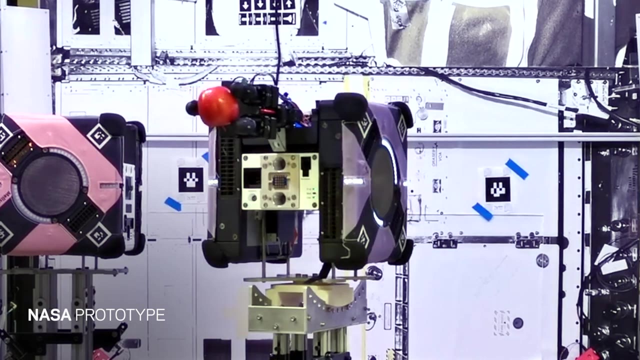 So we've been asking: can we optimize the mechanical design of a robot at the same time as the computational policy with and for each other? And this is where we come to the big, big advances that we've seen in the last five years. 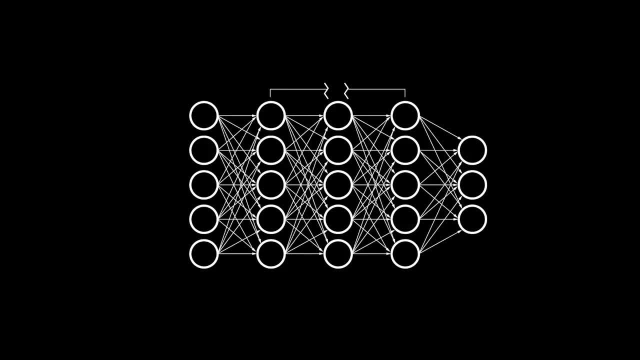 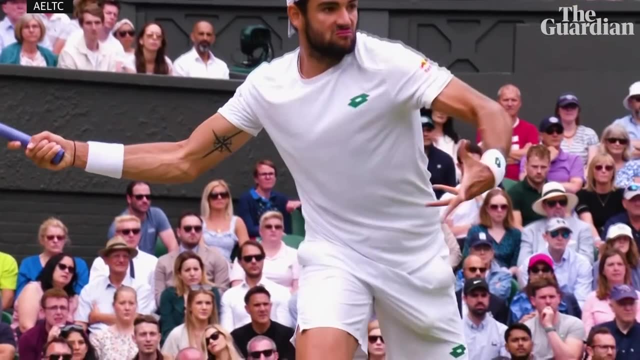 The first is the field of machine learning and reinforcement learning. Some of these modern reinforcement learning techniques are really really well suited for operating in situations where you have imperfect knowledge of the world. You can think of it almost as a muscle memory, right, Every time you hit a tennis ball you don't have perfect knowledge of. 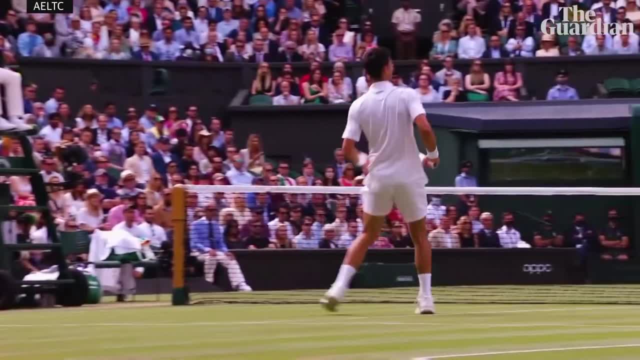 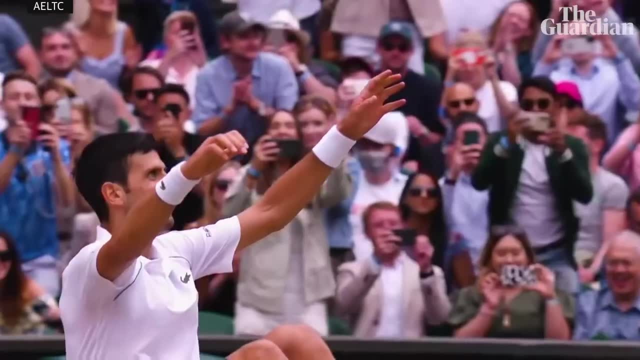 the ball's exact velocity and speed. You get your sensor data which tells you something about the world, and then your muscle memory takes over and says: you know, last time how did the world look like this. These are the actions that I took, and things turned. 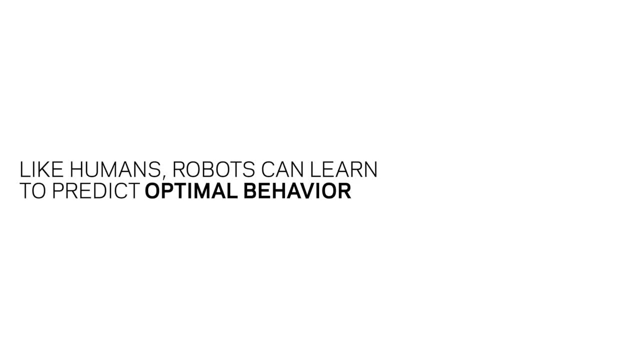 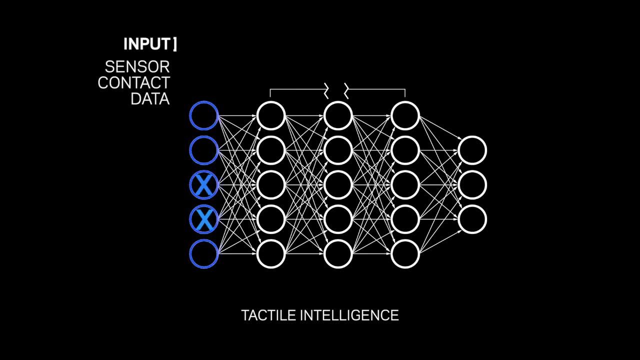 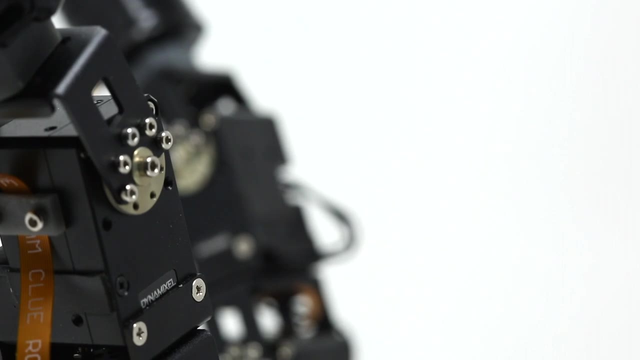 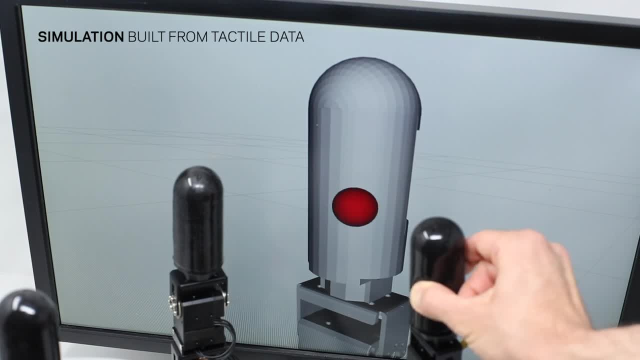 We've been working on this for a long time, So we've been able to build this new neural network with new sensors. We've been working on this new neural network with new sensors. We've been working on this new neural network and reinforcement learning methods to mine. 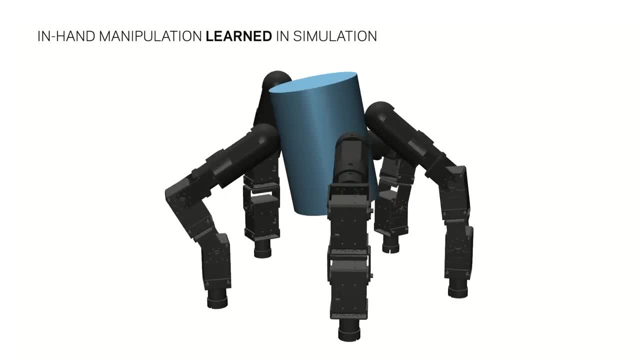 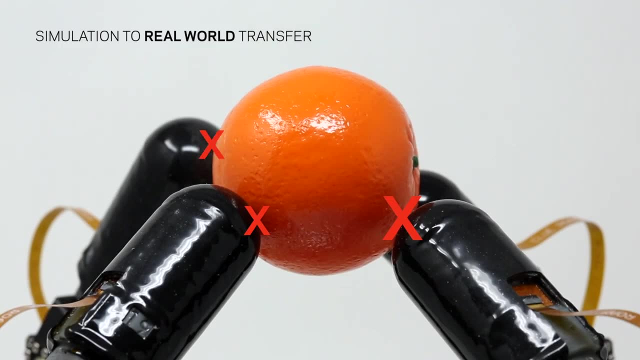 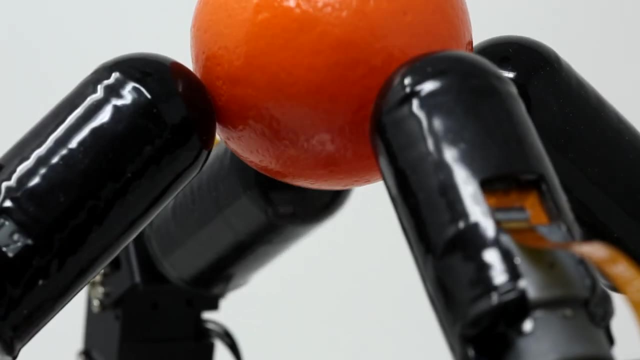 it for the information that's relevant to manipulation, And all of those can be designed to react appropriately to unforeseen circumstances, which is the definition of intelligence: right to do the right thing when you are faced with a situation that hasn't been predicted. 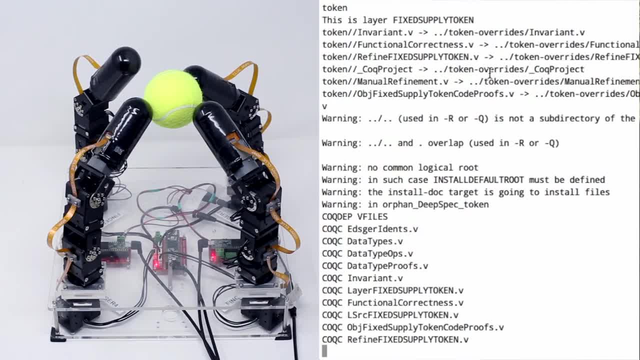 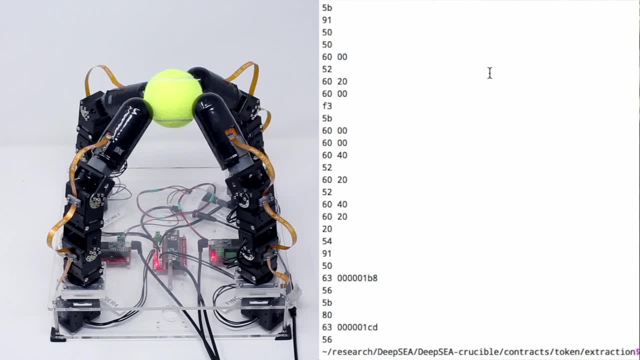 What we'd like to do is move away from the real world, from the own experience, from the actual reasoning, But what we'd like to do is increase the potential and the ability to make decisions with these sensors, the paradigm where one group designs the mechanism and then kind of throws it over the wall and says: 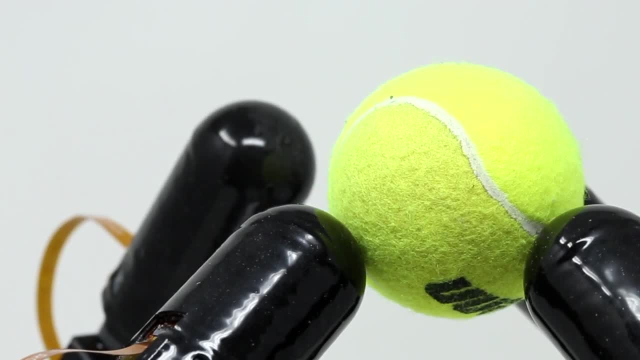 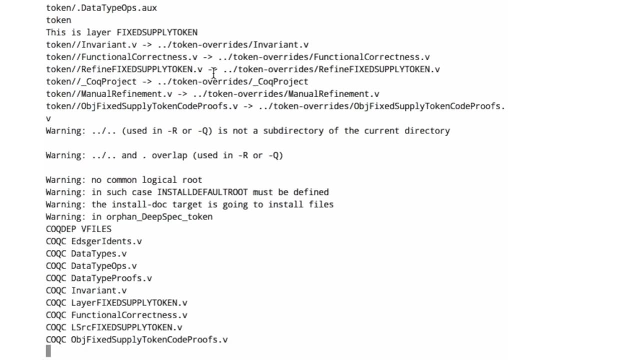 hey, computational people. you take it from there. the mechanism looks about right. it should be able to do everything. it's just the software problem from now on. and then you get the software people saying, oh, it's the mechanism that's letting us down. our software is very intelligent. what we're. 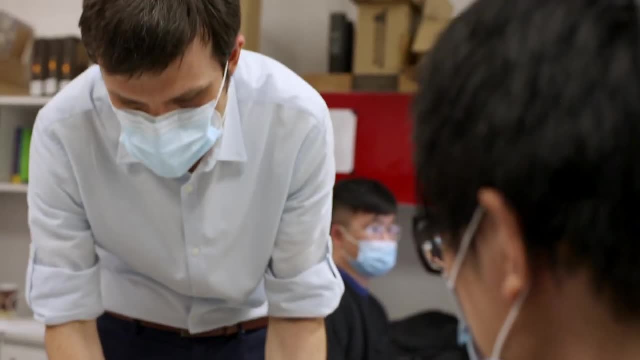 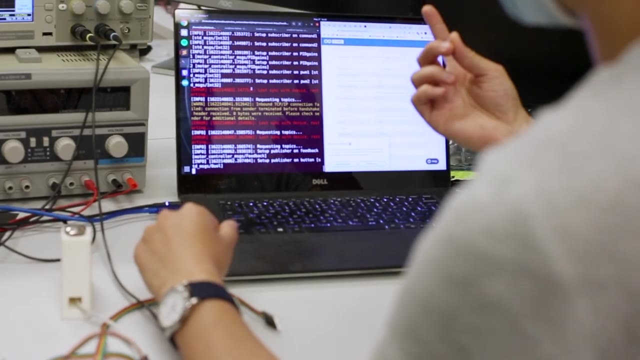 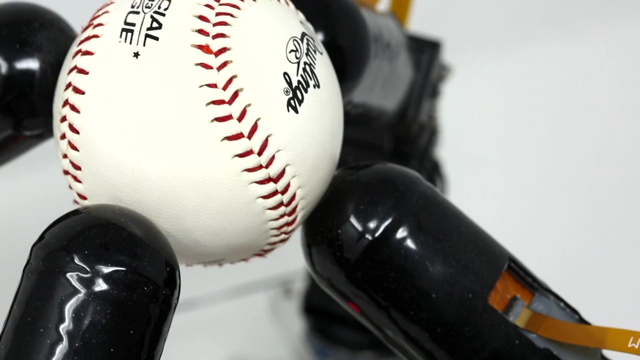 saying is that if you think about them as a whole, that's when we're going to see a very noticeable improvement in performance. because when you talk about embodied intelligent agents, there is really no choice but to look at the mechanism, the sensing suite and the computational aspects- all of them. together. So listen, the rumors are true. There are college majors out there that are both easy and they also lead to high paying jobs. And if you pick the right major, you can actually enjoy your college experience, not be stressed out all the time and then afterwards get a high paying. 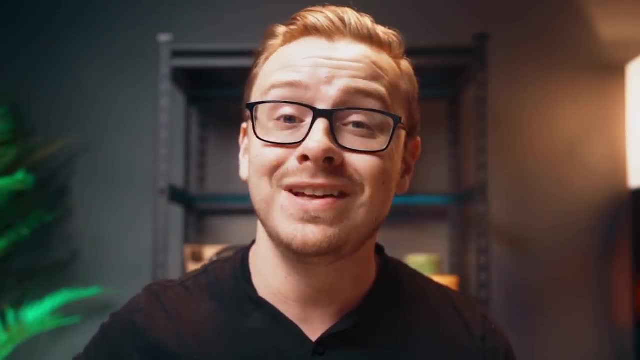 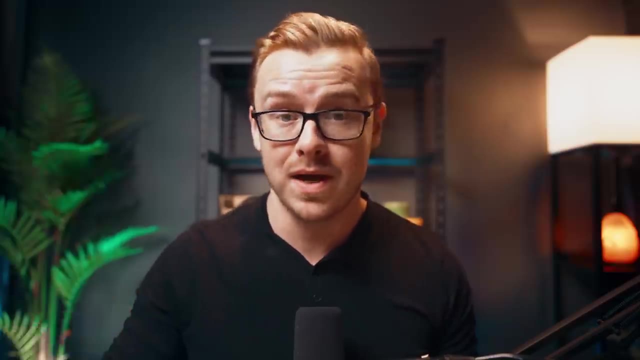 and fulfilling job, And that's why, today, I'm going to be revealing the seven easiest college majors with high pay, And I'm also going to be talking about why they have high pay. So not only will you know seven good ones, but you're also going to recognize other opportunities as well, just in. 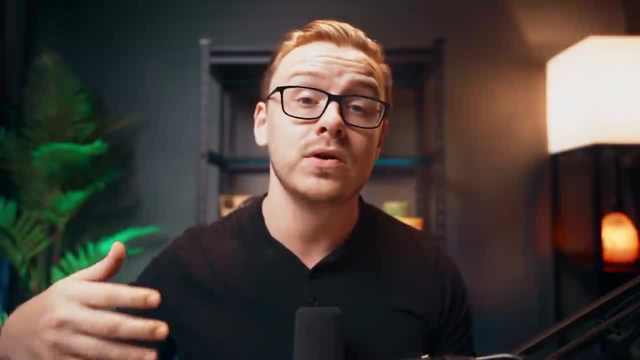 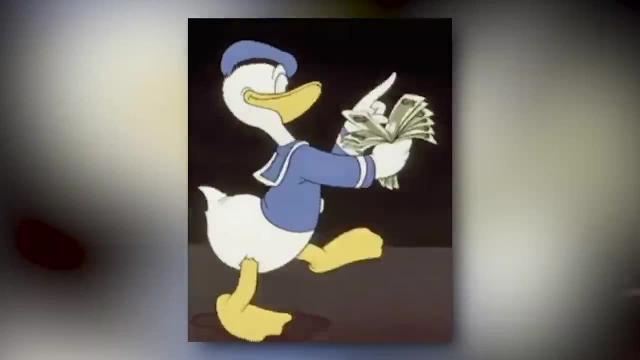 case, one of these don't fit your personality, Because when you choose a career using this simple framework I'm going to lay out in this video, you're going to be 10 times more likely to choose something that is going to pay you well and is also going to make you happy. And I'll let 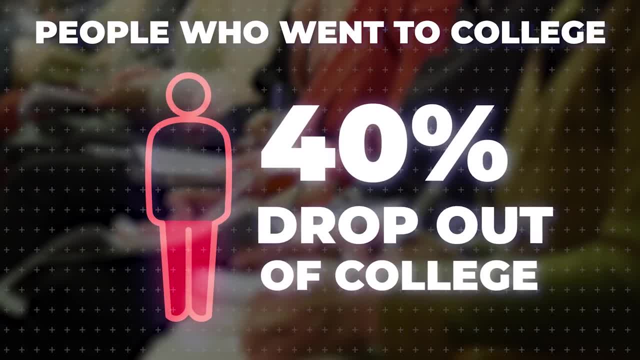 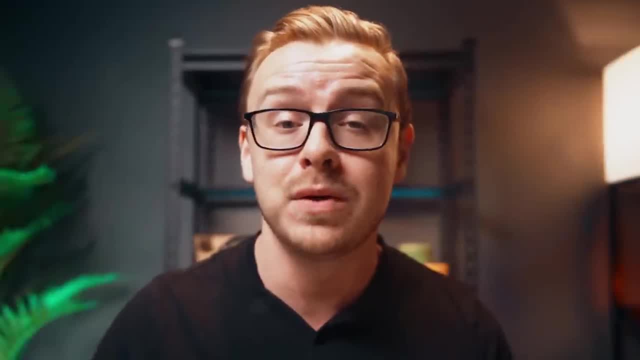 you in on a little secret: 40% of people drop out of college and of the ones that finish, 50% of them regret it. So that means college is a disaster for over half the people who go. But that won't be the case. So let's get started. 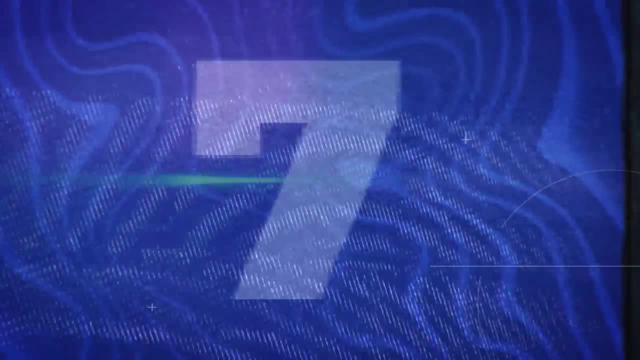 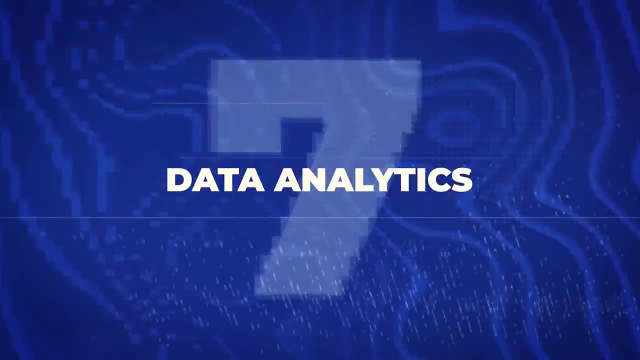 It won't be the case for you as long as you follow along, And number seven on the list is going to be one that is incredibly valuable in the modern world because it's going to deal with data. That's right. With the rise of big data, companies are looking for people who can sift. 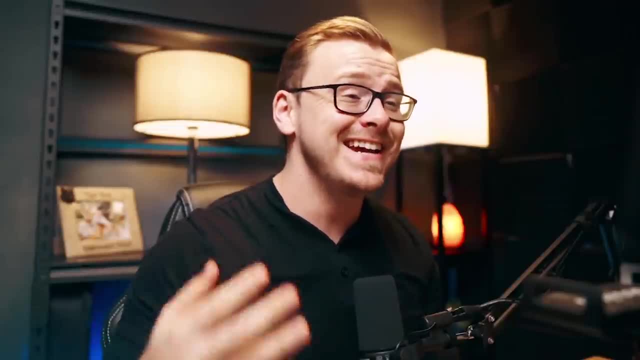 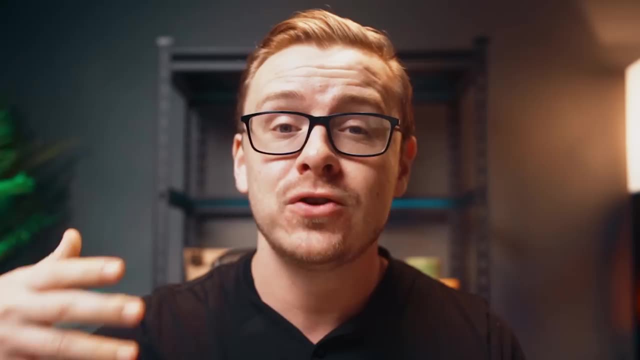 through all of that information and make sense of it And, if you think about it, data is incredibly valuable. So I'm a fan of chess. for instance, And who do you think is more likely to buy a chess set? So let's say, a company is spending a million dollars to advertise a chess set. Who's more? 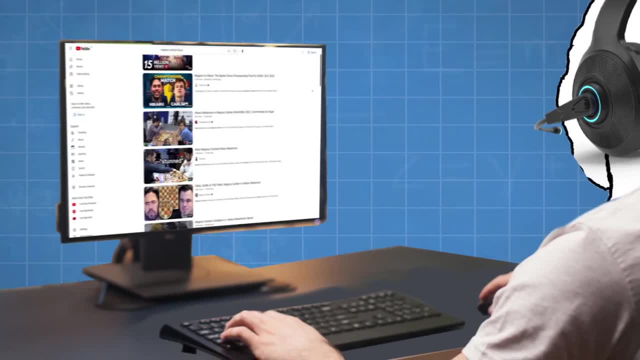 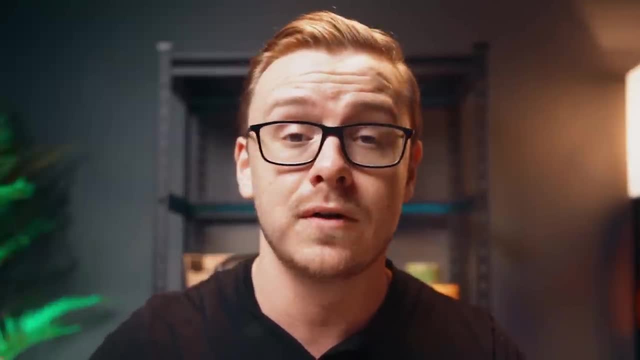 buy something. Somebody who's viewing history is full of Magnus Carlsen and Hikaru Nakamura videos and they've been watching a bunch of Gotham, Chess or Agad Mator videos, And it also shows that they're a fan of the show The Queen's Gambit, or somebody who has never watched or played chess. 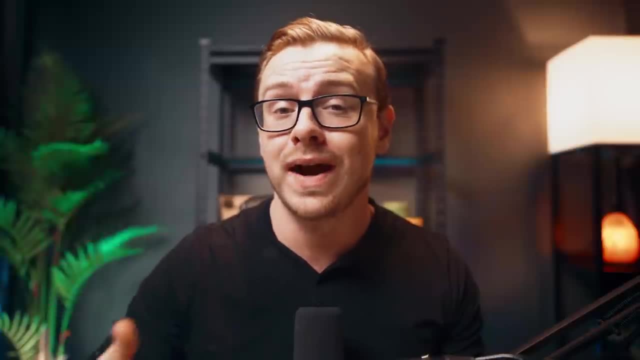 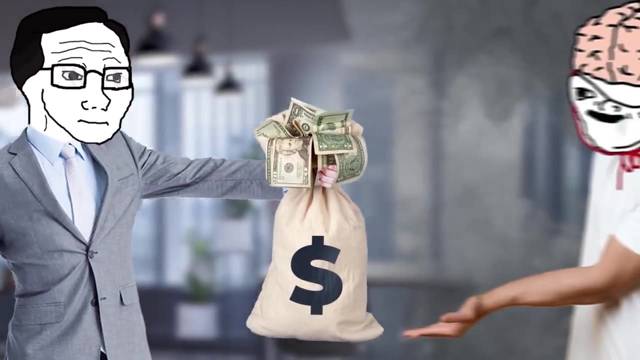 before. Obviously, it's going to be the person who has been interacting with chess, And this is exactly what data is going to tell you. In one case, if the company spent a million dollars on somebody who's never interacted with it, they probably would lose like $900,000..